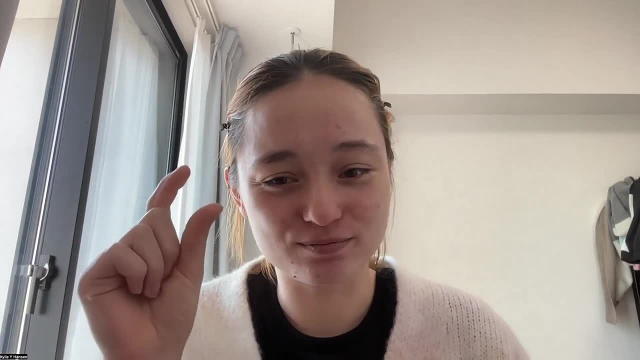 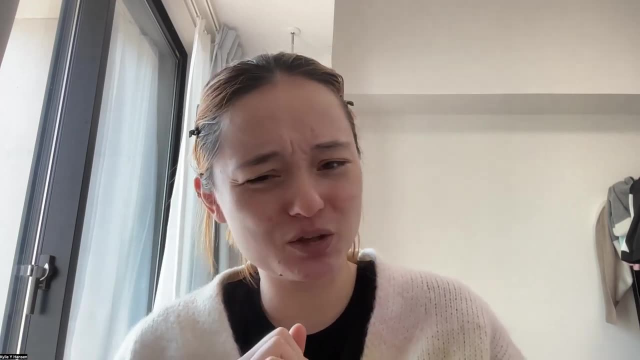 the simplest objects you can analyze. They just look like kind of little points of light on your data frame. You have a data frame with those points of light on it, aka stars, but those points aren't actually points right. They look more like smallish circles. 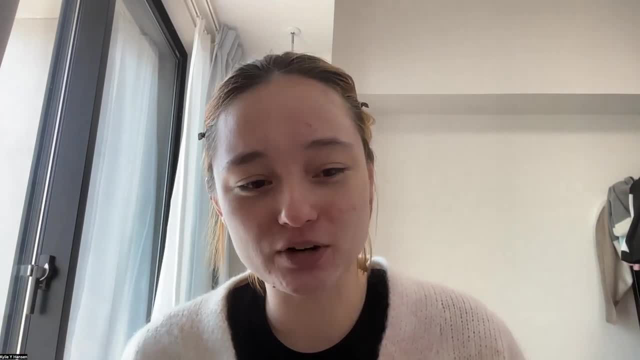 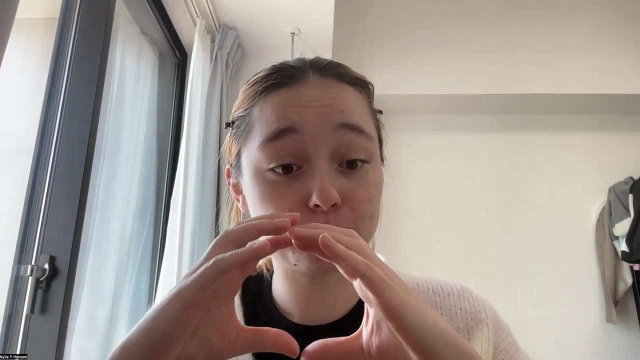 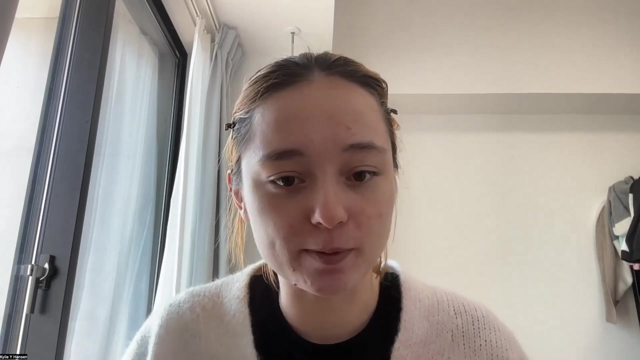 So to measure the entire flux we get from a star, we need to include all the light from that small circle. We can do this by defining an aperture around the light and summing the amount of counts within that aperture. Let's get into the coding So I'm going to share my screen. So before we, 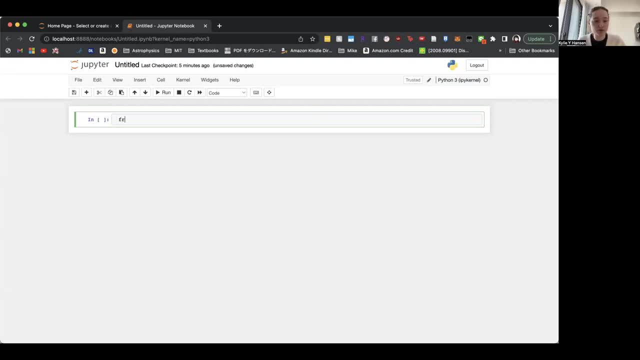 start with the aperture stuff. we'll want to make sure to import a few things. So we're going to import from photos, From PhotUtils, import aperture, photometry and circular aperture. Make sure first of all you have PhotUtils properly installed, And then from PhotUtilsaperture we'll import circular. 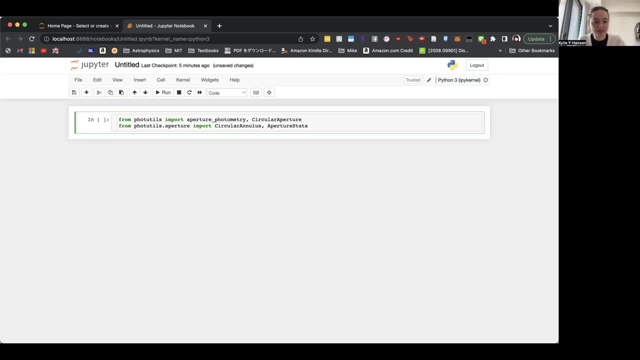 annulus and aperture stats, And then we'll also import math. We're going to be doing some math, Yay, Alright. so we'll go through an example using PhotUtils. Firstly, to define this aperture, we need the center of the aperture as well as the radius of the aperture. So remember: 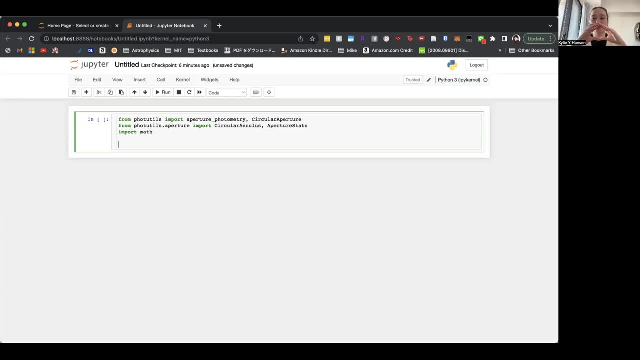 the aperture is surrounding that little circle of light that is our star. So ideally you would find the exact center of your star using a program like SourceExtractor or some other program that you you could use in Python. the common one is SourceExtractor, But we're not going to go into 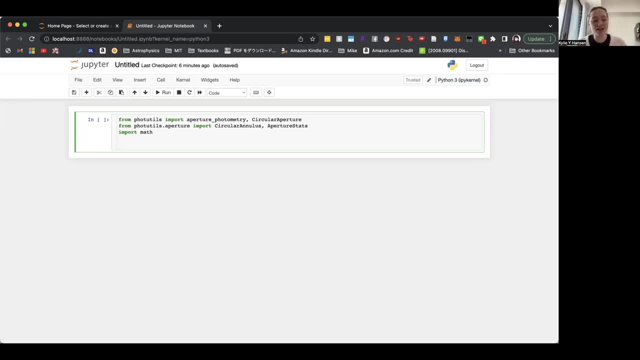 that now, because it's kind of complicated. We're not going to do that right now cuz it's kind of complicated. so we'll just assume that you've obtained the position of your star, or you've estimated it somehow, so you can thus define your aperture as such. so we're going to find a position. 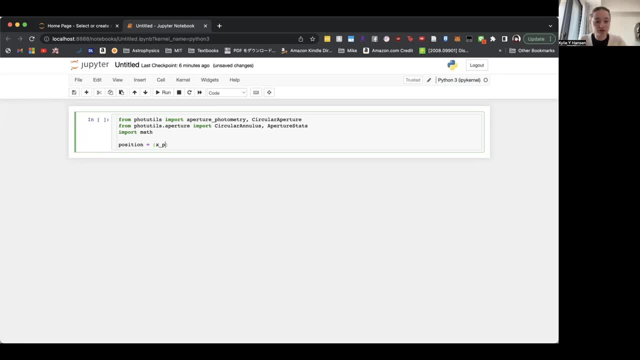 where we have our aperture. so we'll have our position, or x position in our pixel value, and then the y position. so these will be the pixels of your, your frame, and then we'll define a radius for that aperture, for how big it is, and we'll just say it's like three pixels. so this is. 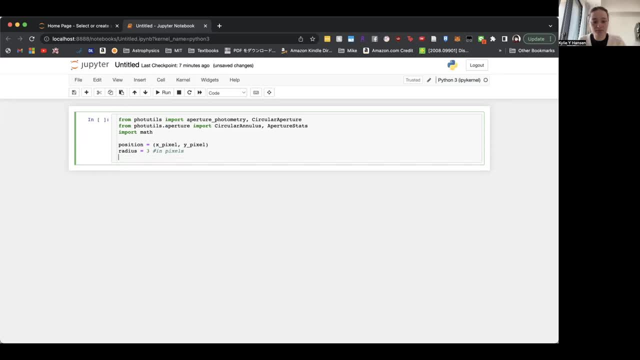 the radius in pixels, okay, and then we'll just define our aperture as a circular aperture with the position and then the radius. so i should note that you can also do this. you can make lots of apertures at once by just creating a list of these things, so a list of all these positions in this form. so if you turn this, 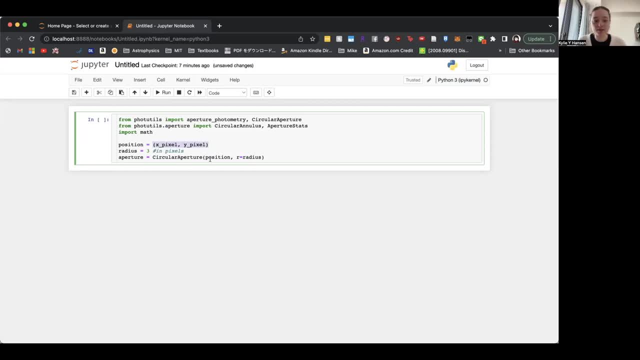 position into a list of these two values. um, then you can make a circular aperture that contains a bunch of different positions in them all with this same radius. so this could be particularly helpful if you want to speed things up. you can create a bunch of different circular apertures. 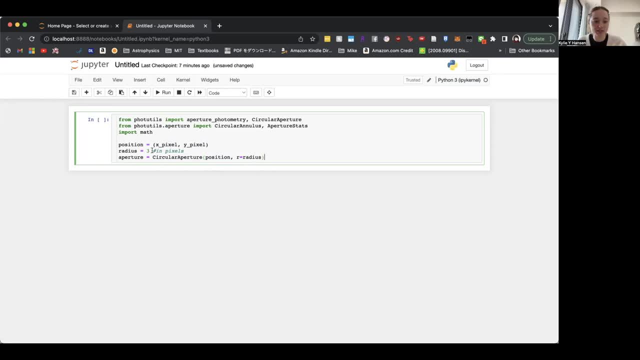 at once, but for now we'll just assume that you have a single position. okay, so then? um, this thing is created, so now i want to sum the counts in size and then, so you can do that by just using the aperture photometer. you can see on the right. 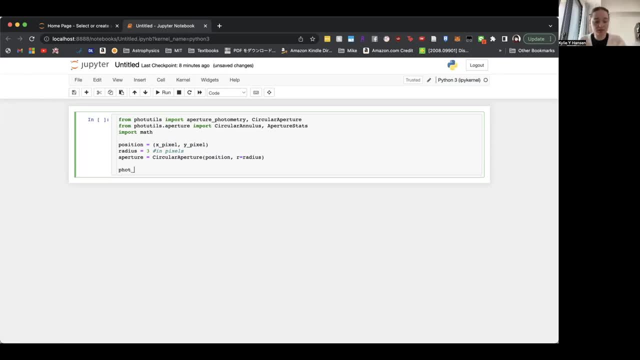 side of that aperture using the aperture photometry function. let's do that. so we'll just call it photo table, because it'll produce a table for us. so aperture, photometry, and then we'll include our data and then the aperture. so data, um, basically, is the data from your data frame. so ideally, 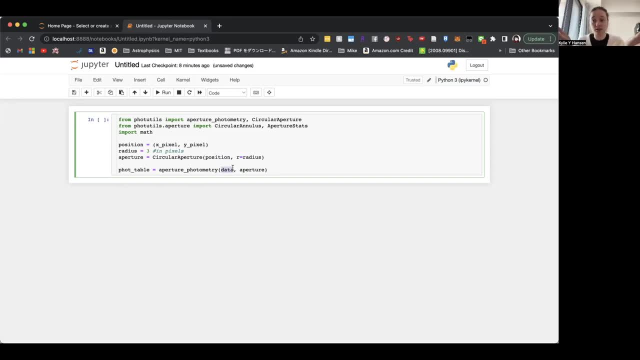 file. so in the fits file you can get the data, which is a numpy array, ideally, and so, um, this here will be the array that includes all of the data from your fits file. okay, so this gives you a table with the aperture sum column. i'll write it out. so the aperture sum column is the sum of. 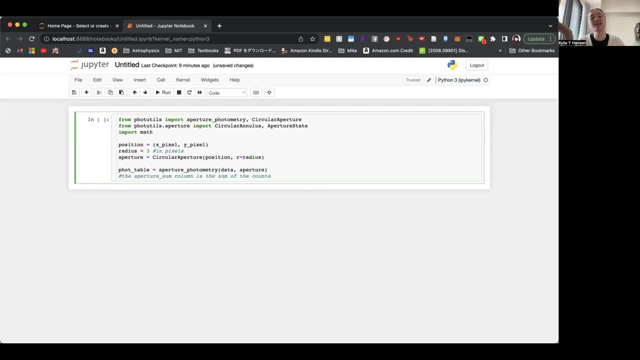 the counts within the aperture. so we can't, unfortunately, use this number directly, because it also includes the counts from the sky itself. so the sky itself, uh, kind of produces some, some kind of light. so unless you're out in space, you'll have to subtract that amount of light that the sky 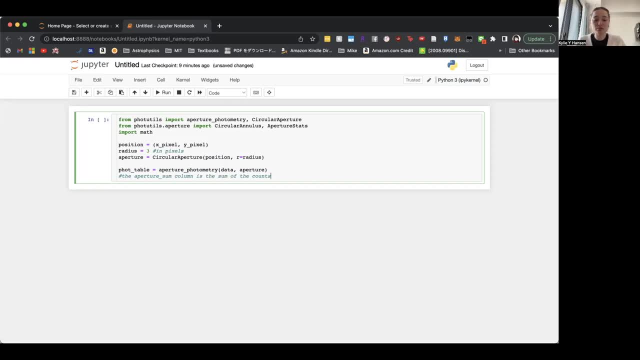 itself emits. so to do this, we will make an annulus. an annulus is basically a donut, so we'll make a donut our way around the sky, and then we'll make an annulus, and then we'll make a donut our way around. 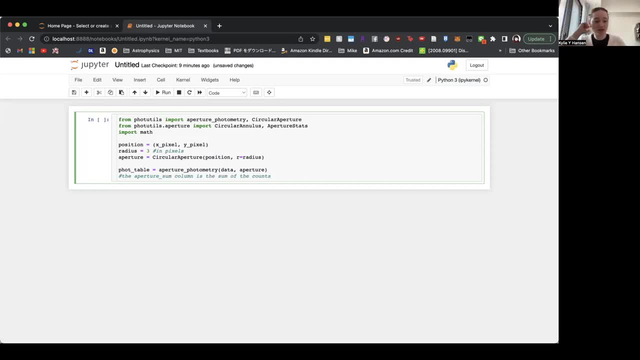 um the space around our aperture to calculate the background light. that's in that area where aperture is. so ideally, you know you want that that donut to be close to where your aperture is, because the background amount of background light you get could shift depending on where. 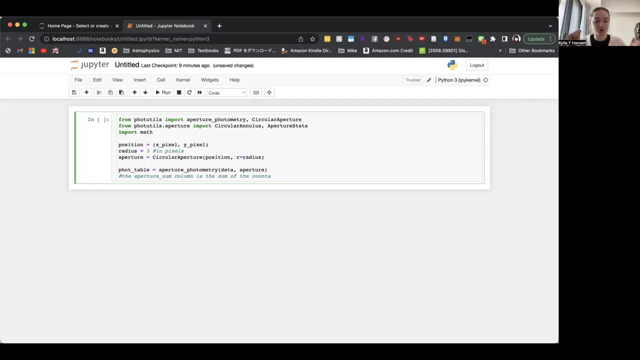 it is in your image. so ideally, we'll make it right by our aperture. the outer edge of this annulus, the outer edge of the donut, is defined by R-out and the inner edge is defined, defined by r in. so we'll see that as i type it here. but remember, so just keep in mind that you. 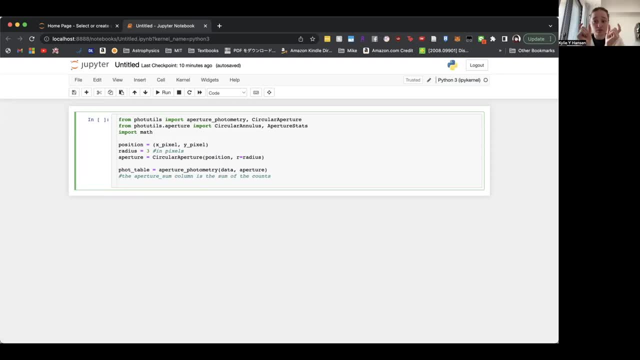 um should set your r in and r out values, but basically setting the width of the annulus to make sure that that annulus does not include any other strong sources such as, like other stars or um, i don't know, maybe you have galaxies in your image or whatever- but making sure to exclude as 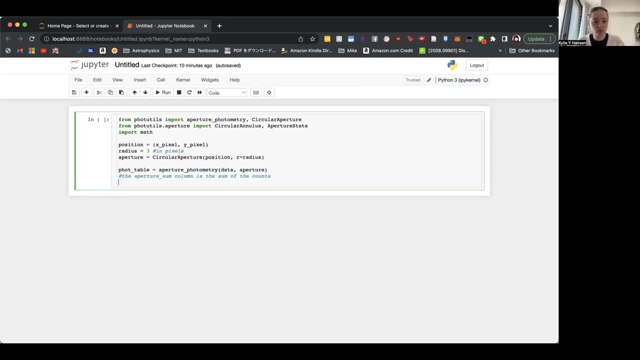 much of that as possible. that's what you want to do, all right, so we'll make the annulus annulus aperture, use the circular annulus function. so we'll want the same position as we had before. and then r in. we'll just give it two random values. since i don't have any data i'm using here. i'm 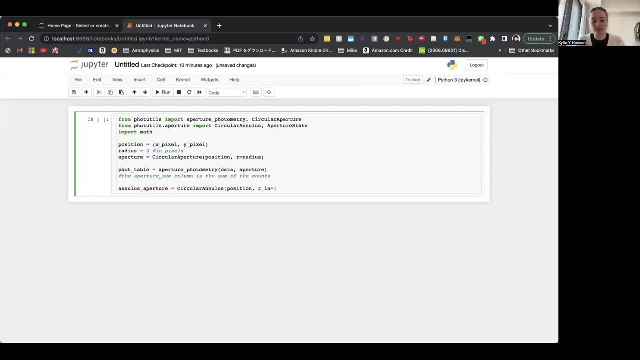 just you know typing this out for y'all, so we'll just say that it's five. so our radius up here for our original aperture was three, so we want it to be at least three or greater. so we'll just call it five. and then the outer edge. 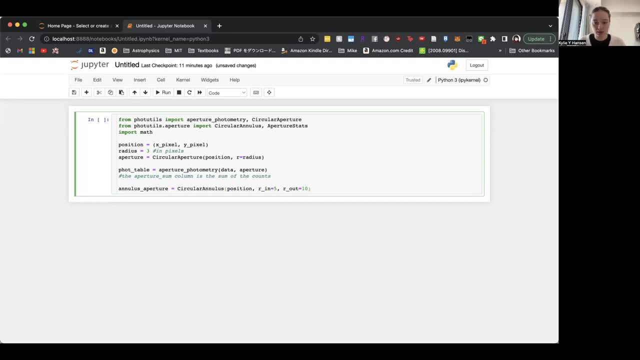 will be ten, for example, or it could be smaller whatever, but however thick it can be without including other stars or other things in the area. so if you have a really crowded field, it might be super small, right? if there's hardly anything in the field, maybe you can include a ton of area. 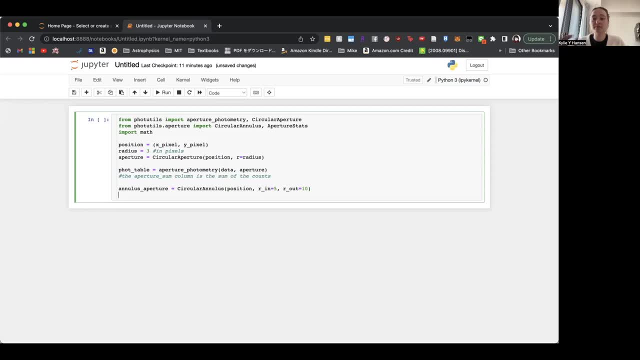 around it, okay, and then we'll want to do some math. so basically we'll do upper steps, aperture stats, so we'll want to do some math on this aperture. so, or the annulus, so we'll take our data and then include our annulus aperture and then we want to take the mean of the background. 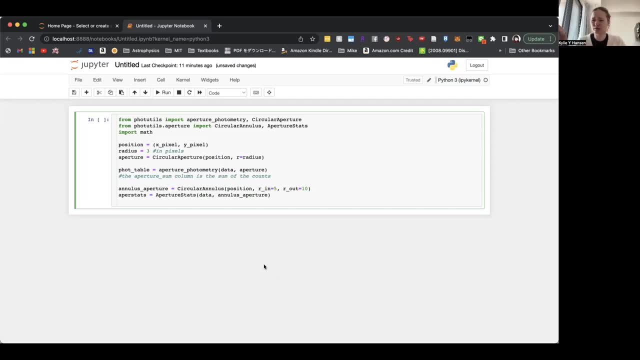 or i guess the median- if there's a lot of outliers, but, um, usually mean or median- and then multiply it by the area of our aperture, not the area you want the area to be right out of that part. so you want to take your aperture and you want to think of you. i believe it's. 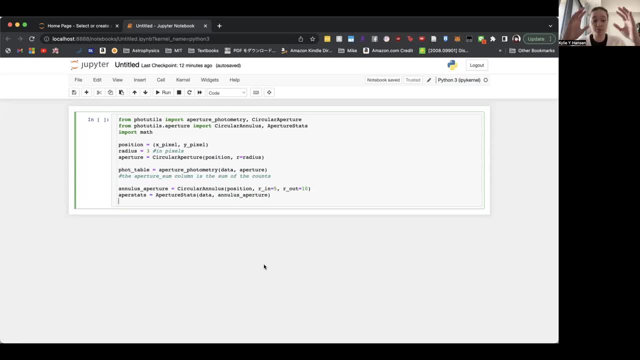 an fitted figureción. there you go, line work out, and then the sine is gonna be the same number, right, so, right now. so now we can put this in the same ratio, not the area of the annulus, the area of the aperture, because you want to get the total. 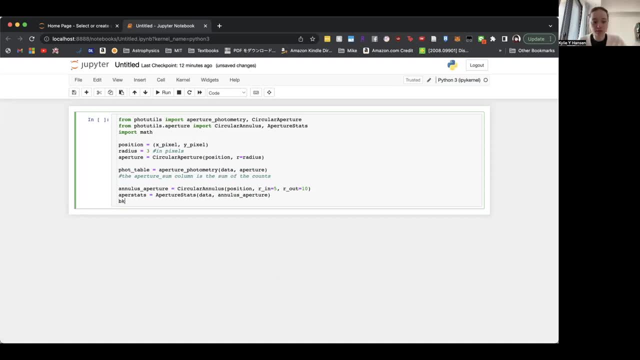 amount of light from within that aperture. so we'll take the. we'll get the, the mean. so aperstats conveniently has a mean, so we'll just take the mean and then the total background will be the mean multiplied by the area of the aperture. so remember, it's not the area of the. 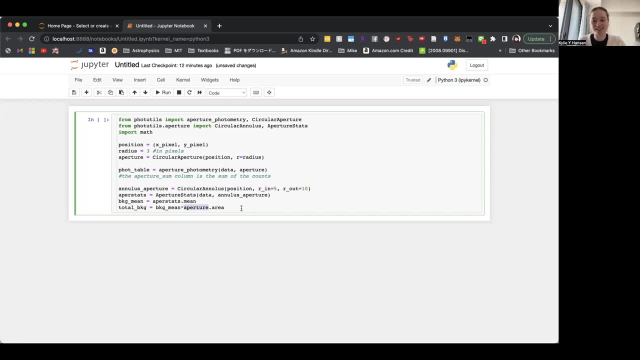 it's the area of the aperture. that's why we're specifying that here. be very careful about that. okay, so now we just need to subtract that background from our aperture sum, so we'll call it background sub. so we'll take the. take the table that we have and remember it's called the. remember the column is called aperture sum. 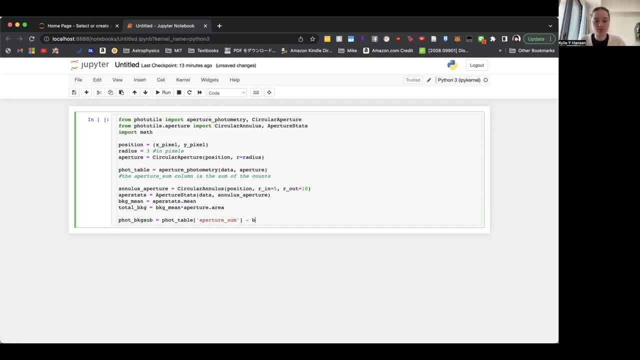 and we'll subtract- oops, subtract- the total background from that. okay, nice, okay. so now we can convert this new sum to what's called an instrumental magnitude. so we use a simple calculation here. so the instrumental magnitude equals um- it's negative 2.5 times the log 10. so 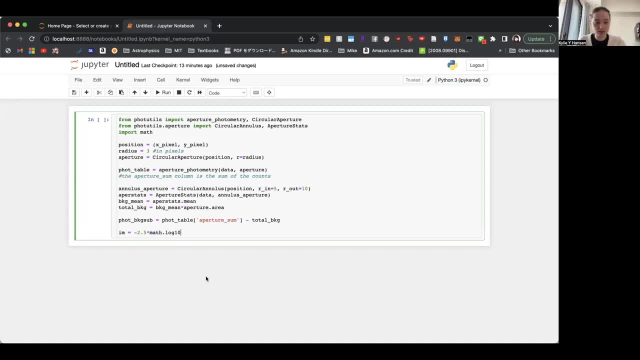 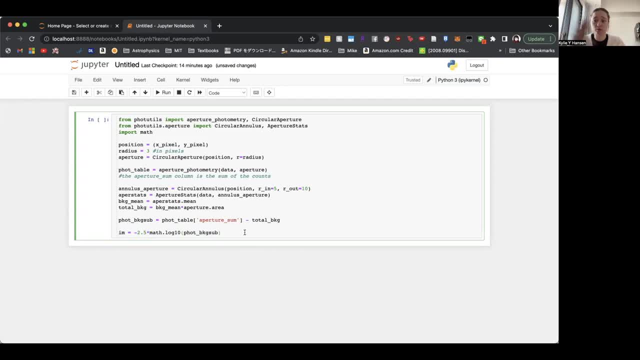 convert to an absolute magnitude which we can use in our science, whatever you choose to do, use in our science, whatever you choose to do, use in our science, whatever you choose to do with this, this number, these numbers, um we with this. this number, these numbers, um, we. 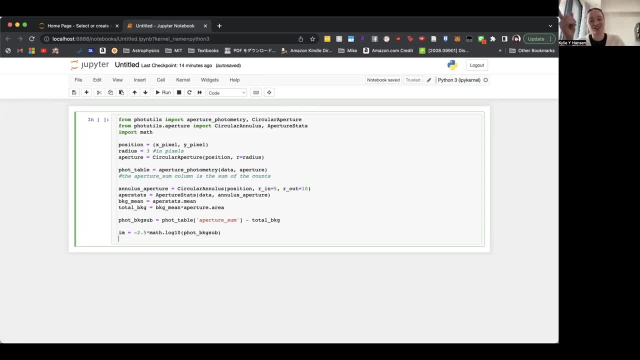 with this. this number, these numbers, um, we want a number we can actually use. so want a number we can actually use, so want a number we can actually use, so remember those standard stars that we remember those standard stars, that we remember those standard stars that we discussed in the previous video. 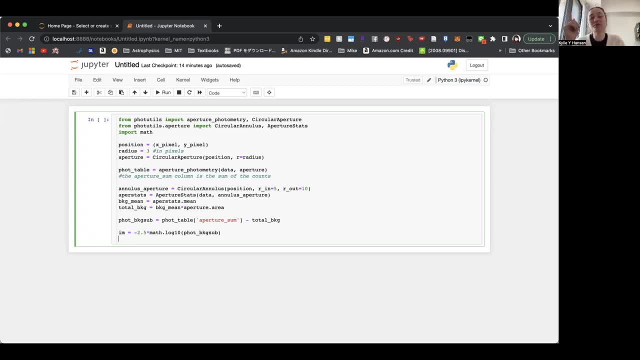 discussed in the previous video. discussed in the previous video, episode two. hopefully you remember those episode two. hopefully you remember those episode two. hopefully you remember those and hopefully there are a few of them in, and hopefully there are a few of them in and hopefully there are a few of them in your frame. or took other frames with. 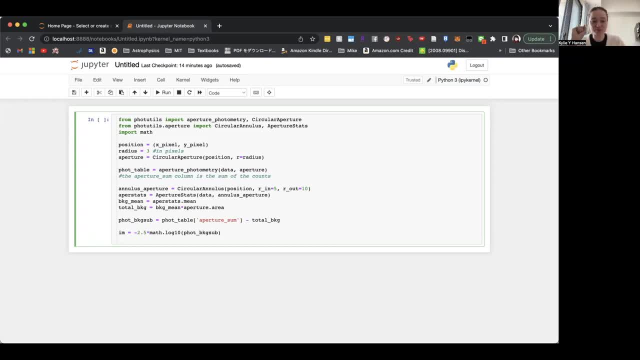 your frame or took other frames with your frame or took other frames with them. so hopefully you have some standard them. so hopefully you have some standard them. so hopefully you have some standard stars. what you'll want to do is do this: stars. what you'll want to do is do this: 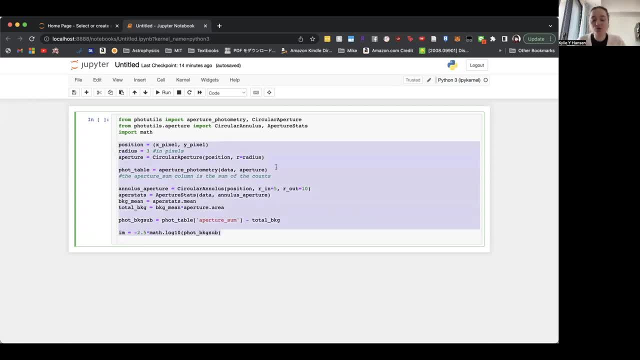 stars. what you'll want to do is do this process, do this process for a bunch of process, do this process for a bunch of process, do this process for a bunch of standard stars and then plot them standard stars, and then plot them standard stars, and then plot them against their absolute magnitude. so against their absolute magnitude, so against their absolute magnitude. so standard stars are standard because they standard. stars are standard because they standard. stars are standard because they have a known magnitude, an absolute, have a known magnitude, an absolute, have a known magnitude, an absolute magnitude, and those magnitudes will vary. 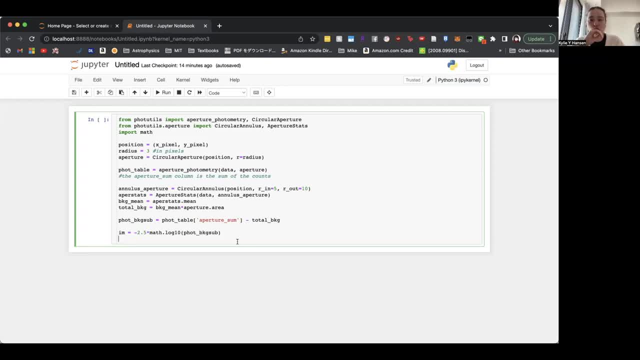 magnitude and those magnitudes will vary. magnitude and those magnitudes will vary based on the color. so you'll want to. based on the color. so you'll want to. based on the color, so you'll want to choose a color that matches the filter. choose a color that matches the filter. 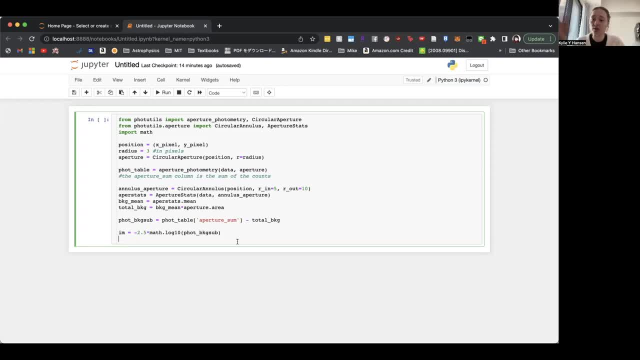 choose a color that matches the filter of CCD that you used, so CCDs will have of CCD that you used, so CCDs will have of CCD that you used. so CCDs will have various filters. an example could be B: various filters. an example could be B. 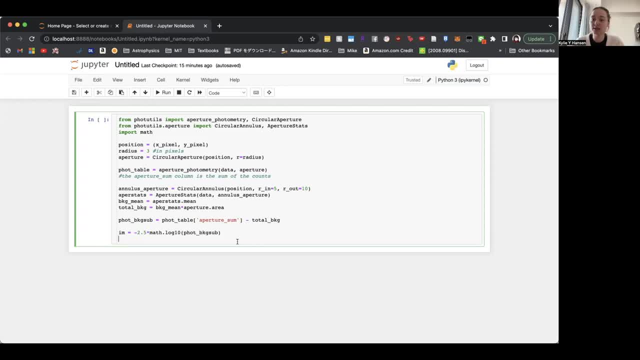 various filters. an example could be B filter or V filter, whatever color filter filter or V filter, whatever color filter filter or V filter. whatever color filter it is using, you'll want to look up the it is using. you'll want to look up the it is using. you'll want to look up the absolute magnitude of your standard. 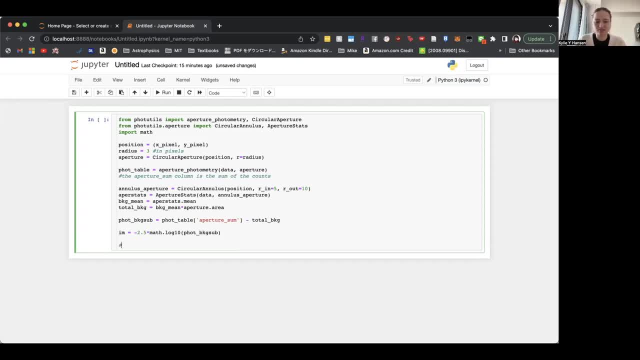 absolute magnitude of your standard. absolute magnitude of your standard stars in that filter and you can use a stars in that filter. and you can use a stars in that filter. and you can use a database like when I use a SIM bad. so database like when I use a SIM bad. so 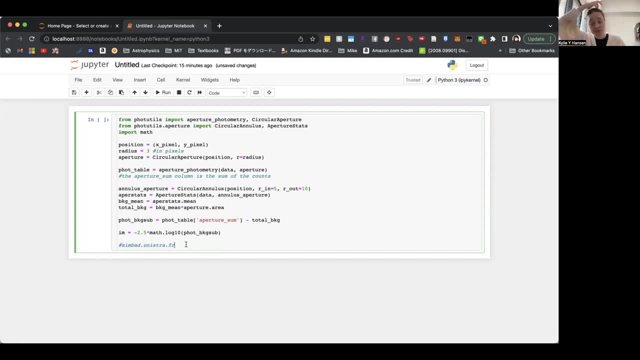 database, like when I use a SIM bad. so this is a database that I've often used. this is a database that I've often used. this is a database that I've often used to look up stuff. so you can use SIM bad to look up stuff. so you can use SIM bad. 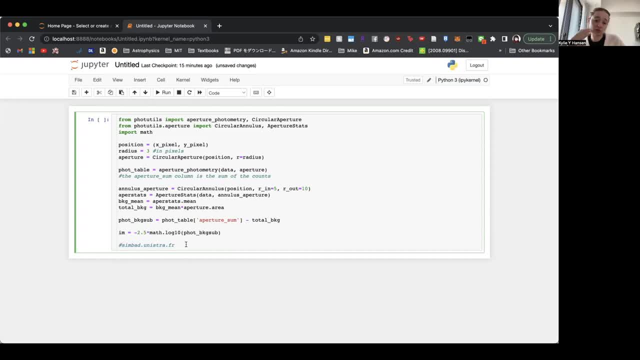 to look up stuff. so you can use SIM bad to look up the absolute value in various, to look up the absolute value in various, to look up the absolute value in various colors. but you'll want to, you know look colors. but you'll want to, you know look. 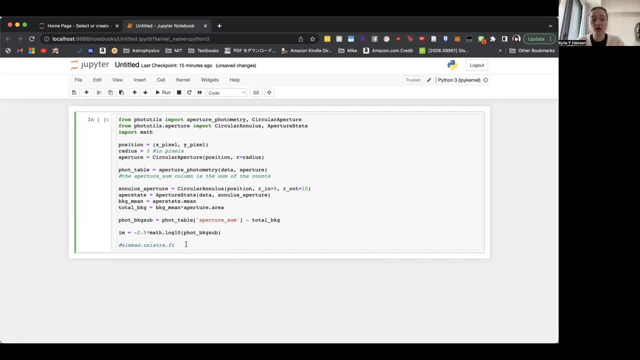 colors. but you'll want to, you know, look those up for your standard stars and those up for your standard stars, and those up for your standard stars, and then you'll plot them. so plot them it'll. then you'll plot them, so plot them it'll. then you'll plot them. so plot them, it'll make like a line, hopefully, so it'll. 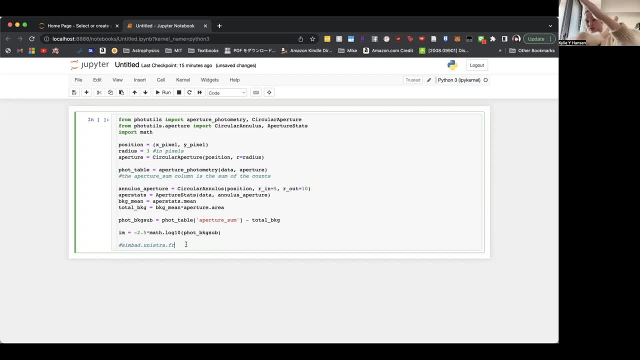 make like a line, hopefully. so it'll make like a line, hopefully. so it'll have the instrumental magnitude verse or have the instrumental magnitude verse, or have the instrumental magnitude verse or instrumental magnitude, and then the instrumental magnitude, and then the instrumental magnitude and then the absolute magnitude, so it'll look like a 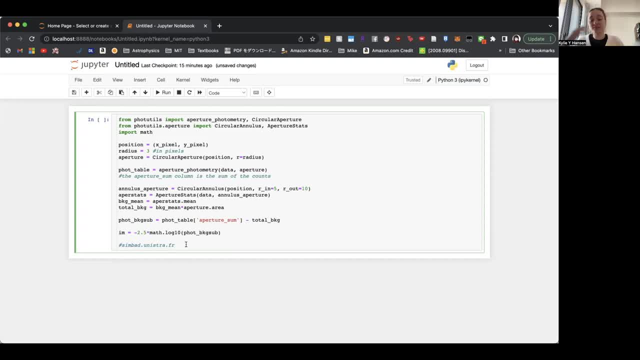 absolute magnitude. so it'll look like a absolute magnitude, so it'll look like a line, and once you have that plot, you can line. and once you have that plot, you can line. and once you have that plot, you can fit the points with that line, using any.